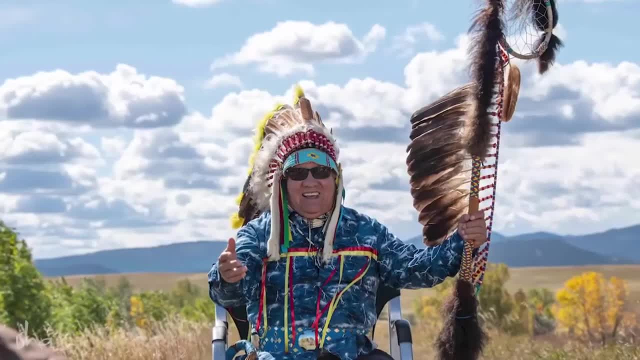 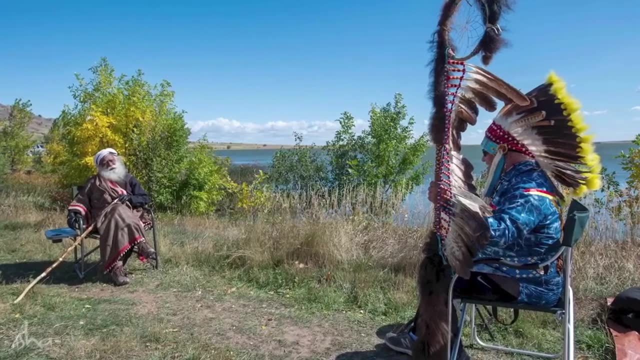 by agents of the US authorities, receive federal subsidies and grants. The US government recognizes the rights of these tribes to self-rule, self-determination and upholds their sovereignty. Sovereign nations have the right to form their own government, to adopt and enforce laws. 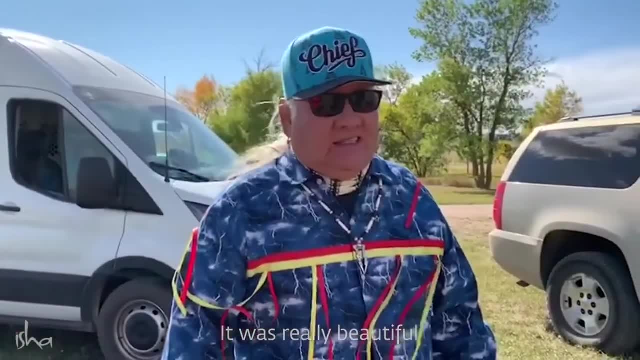 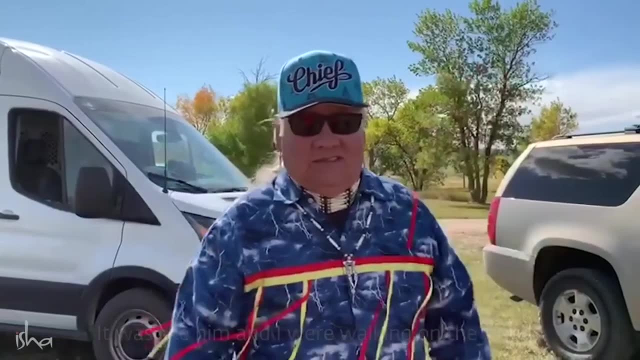 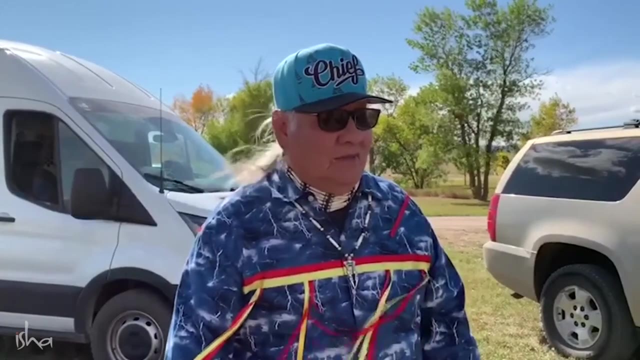 to establish taxes, to assign tribal status, to license and regulate almost all types of activities and to act according to the laws of the state. Tribal courts are active in most reservations And law enforcement. Legally, Indian reservations have practically the same rights as the states of the United States, Just like the states. 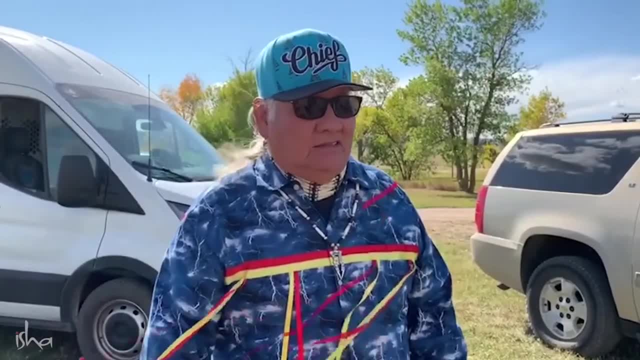 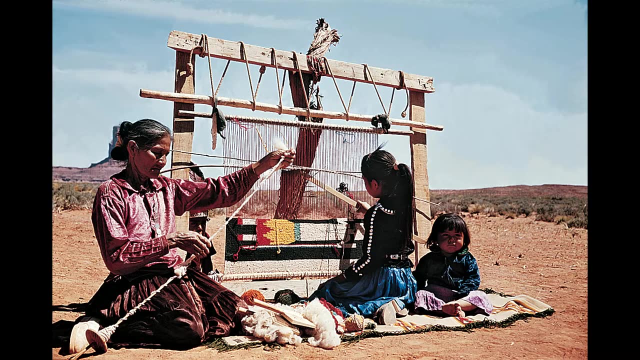 they cannot enter into official relations with other states, wage war and mint coins. The largest Indian tribes today are the Cherokee, the Navajo, the Sioux, respectively, and the Chippewa Indian tribes have the most important human rights. and most of which are war crimes. The state is the most important part of the country. For example, the states of New York and San Francisco are supposed to be the most important European and foreign state For the United States. there are many different states of the. 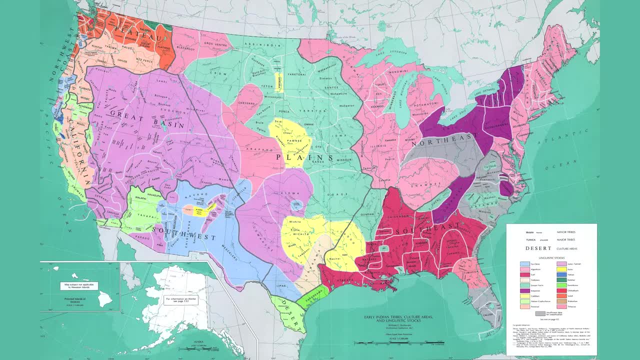 world, especially the United States. several major states are the best and major states in the United States One, the United States, for instance, is the largest Indian land. the United States Indian tribes now control about 2% of the territory of the United States Reservations. 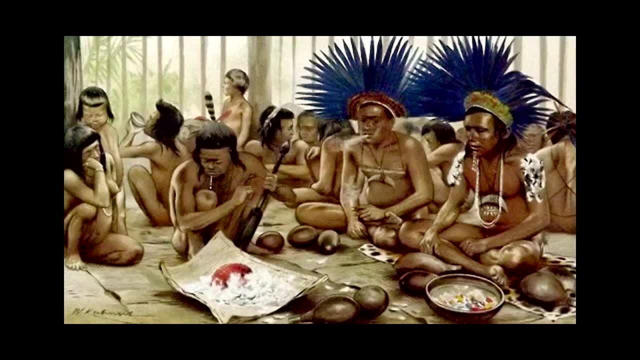 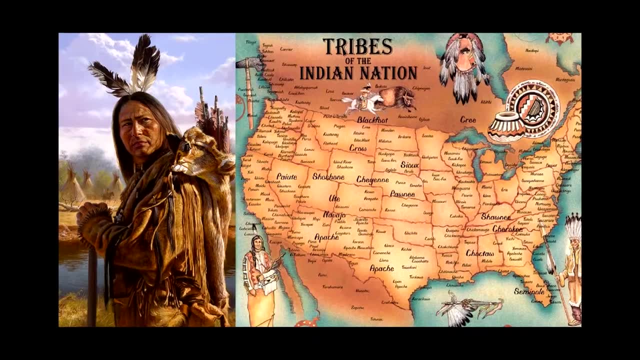 have been formed on these lands. Some reservations are limited to 1 acre. More than a third of US Indians now live on reservations. a third of them are located in Alaska. The average age of an Indian is 29.7 years, which is noticeably less than the age 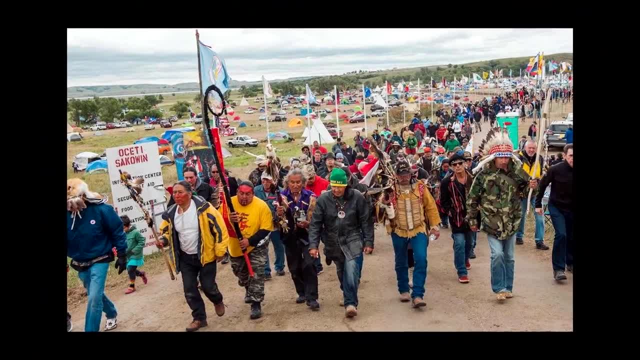 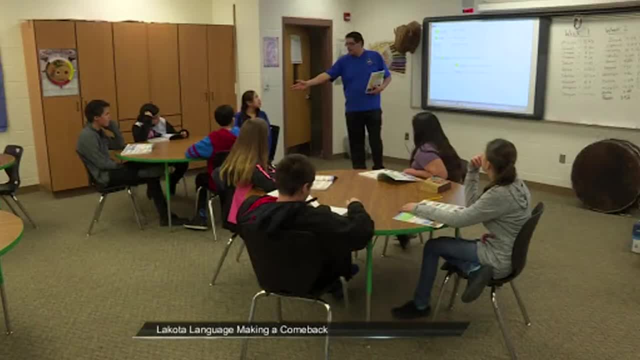 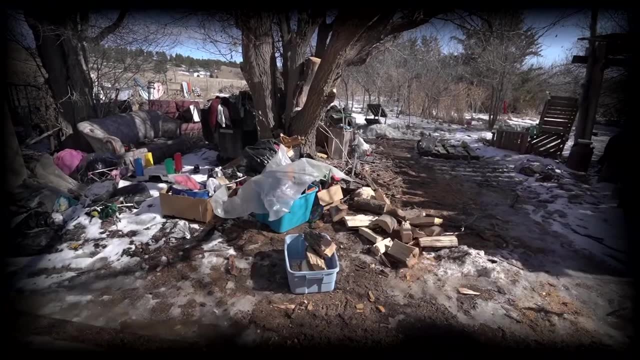 of the average American Indian families have more children than the US average. At the same time, 66% of Americans and only 55% of Indians are residential property owners. Indian houses are much cheaper than the national average In 2009,. 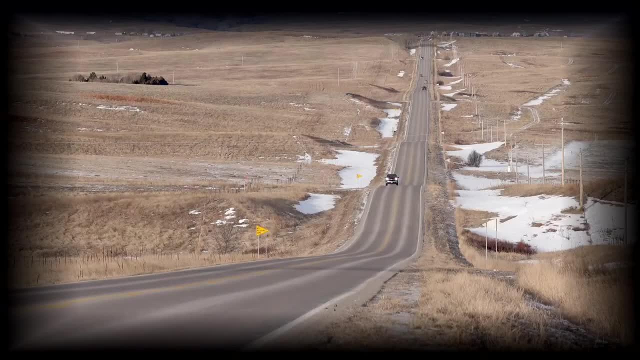 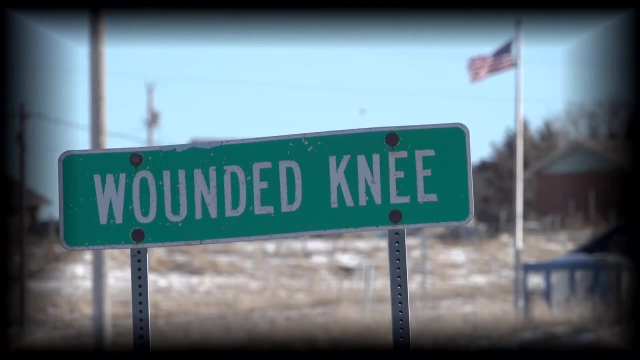 23.6% of Indians lived below the poverty line. The national average, this figure was 14.3%. Despite the fact that Native Americans enjoy significant incentives for admission to higher education and education, the average Indian population in the United States is about. 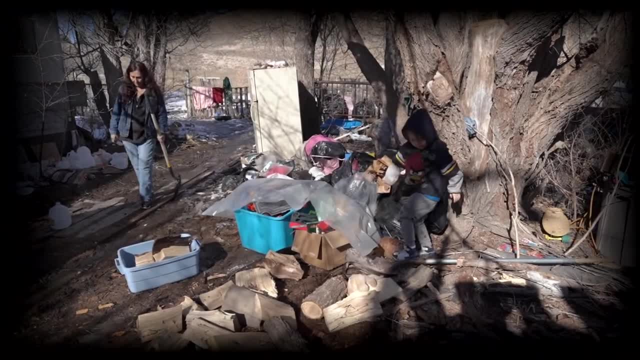 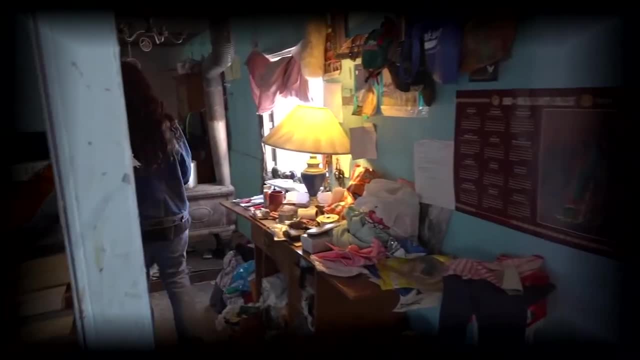 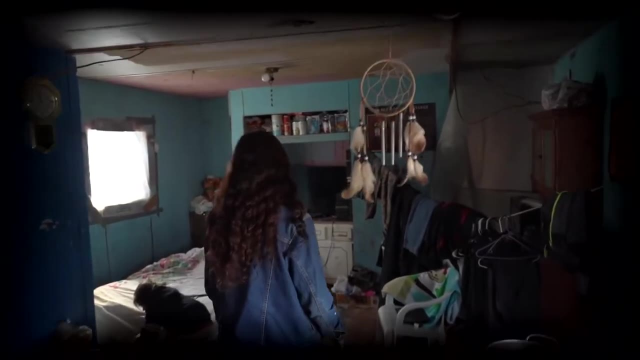 50% less than that of the American population. 28% of Americans have a college degree, compared with only 16% for Indians. According to long-standing statistics from the US Department of Justice, American Indians are twice as likely as the rest of the United States to become victims. of violent crime. There are many more alcohol and tobacco abusers among Indians than in the United States as a whole. Approximately 21% of Indians are in the state of Alabama. going from the United States to Florida, The state of Alabama is the state of Indiana and the state of Florida is the.